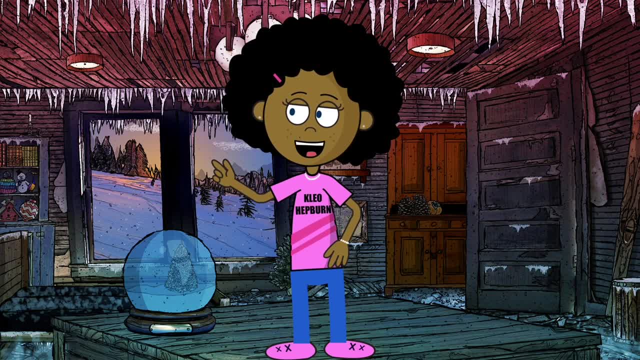 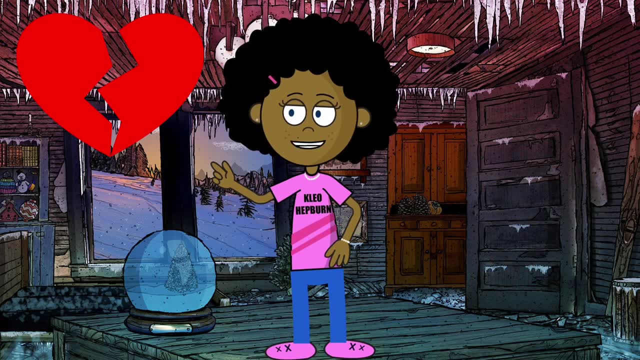 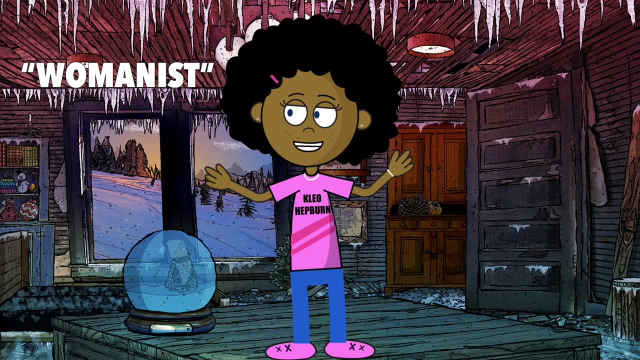 After careful consideration she got an abortion. Later on she got married and had one daughter. Eventually she unfortunately divorced her husband. During their relationship they were being racially abused. in Mississippi In 1983, Walker coined the term womanist in her collection In Search of Our Mother's Gardens, which means a black feminist or feminist of. 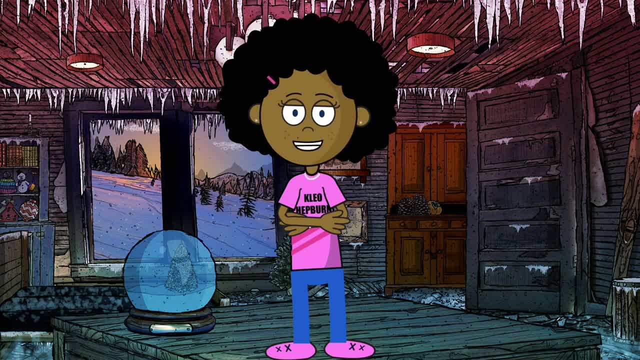 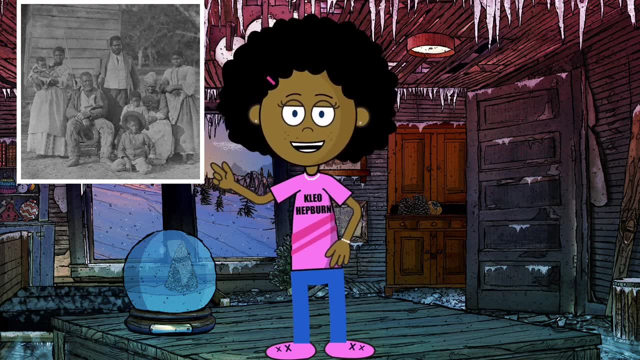 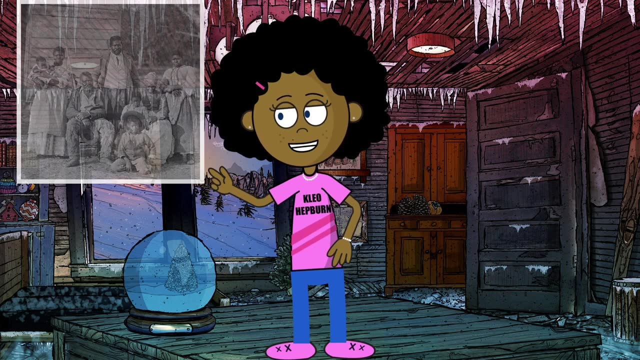 colour. Now we are going to look at the socio-historical context. Black people were treated very badly. Just because slavery had been abolished did not mean that black people were treated equally to whites. Between the time of 1910 and 1940, black people were treated appallingly. There were segregation. 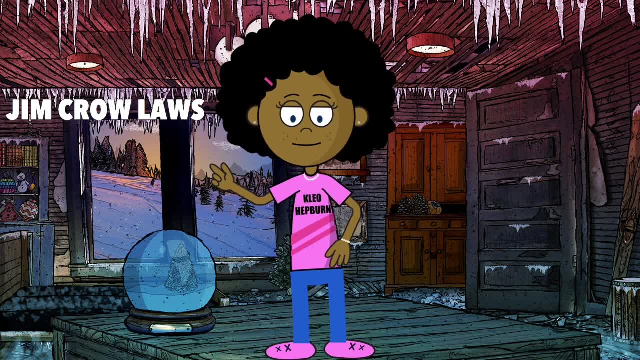 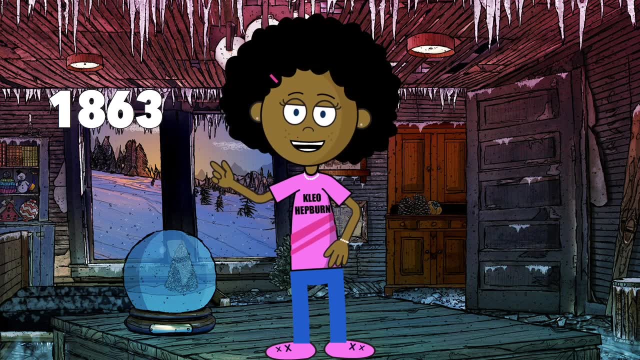 laws that meant that black people didn't have the same rights that white people had. The novel is set between 1910 and 1940. Slavery ended in 1863. Blacks were freed from slavery and began to enjoy greater rights as citizens, though full recognition of their rights remained. 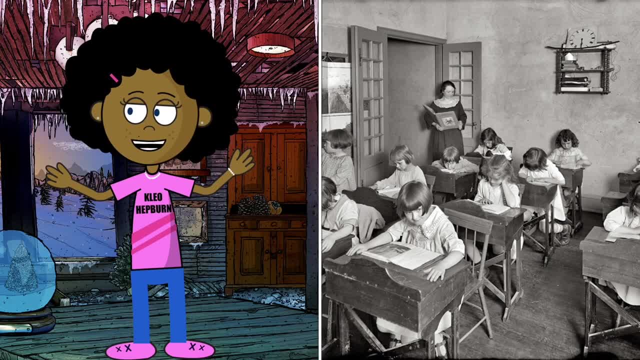 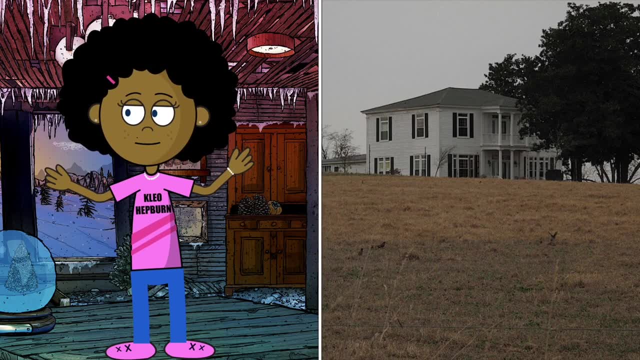 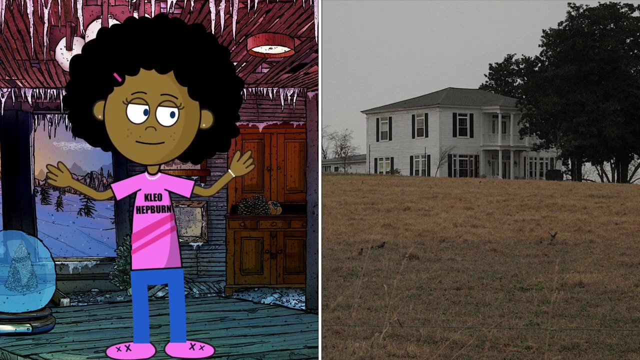 a long way off. Most black children had not attended school before the census and white children were much more likely to have attended. So the members of a typical African American family at the start of the 20th century lived and worked on a farm in the south and did not own their home. Children in these families. 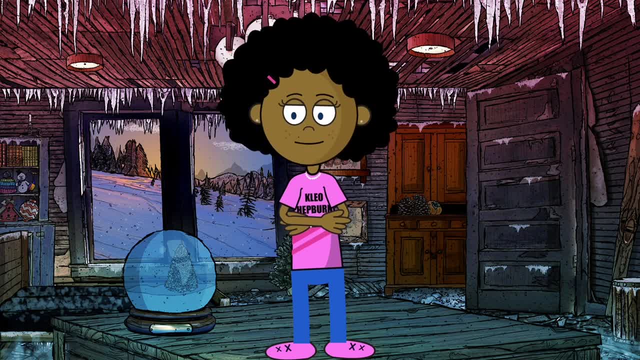 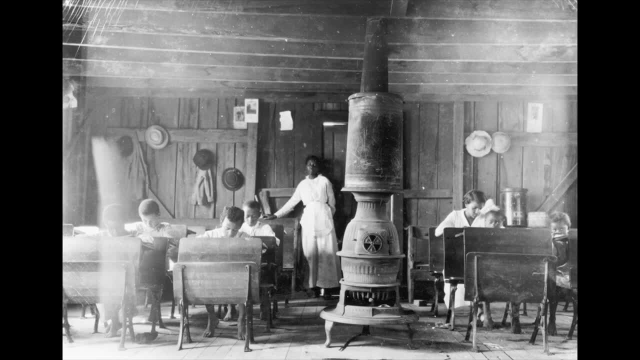 were unlikely to be in school. even at very young ages, Black people grew cotton and many were farmers. They were allowed to go to school, but the school systems were very bad. There were no improvement in resources. as they were pumped into white schools, Black people were. not allowed to go to school, but the school systems were very bad. There were no improvement in resources as they were pumped into white schools. Black people grew cotton and many were allowed to go to school, but the school systems were very bad. There were no improvement. 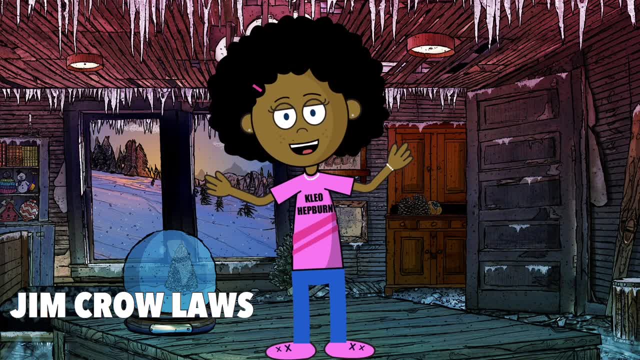 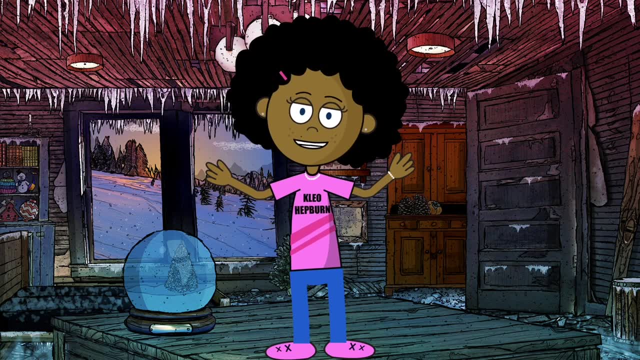 in resources as they were pumped into white schools. Jim Crow Laws were a collection of state and local statutes that legalised racial segregation. It was between 1877 and at the beginning of the Civil Rights movement. in the 1950s, There were different rules in different states. An example is that black and white people